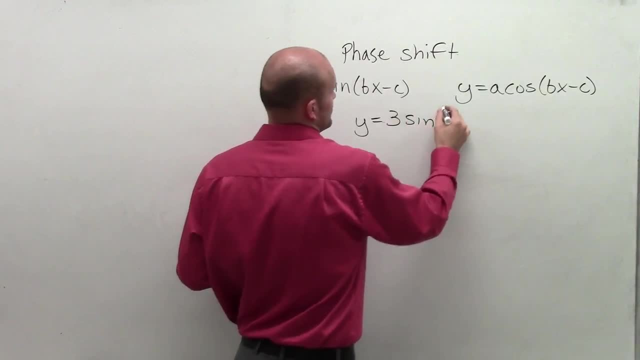 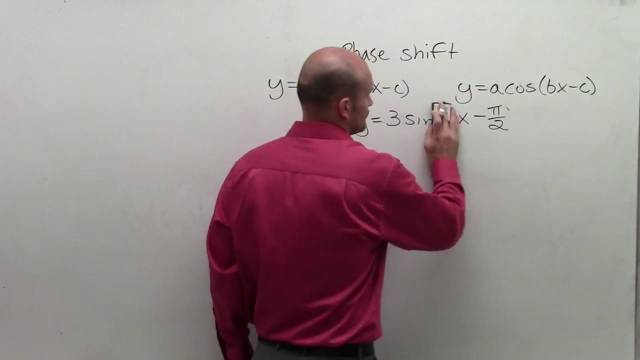 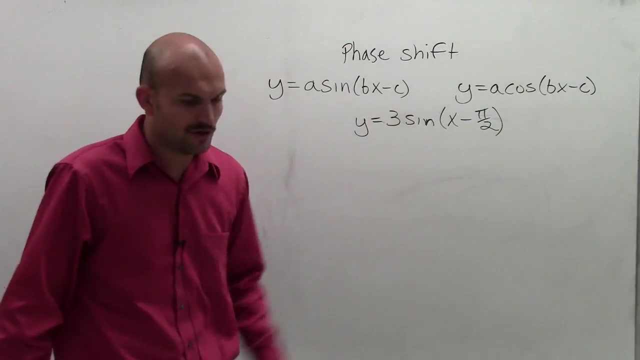 that doesn't work. y equals 3 sine Of 2x minus pi over 2.. No, I'm sorry, y equals sine times x minus pi over 2.. Now, when looking at a function like this, we know that 3 is going to be our amplitude, But we look at: 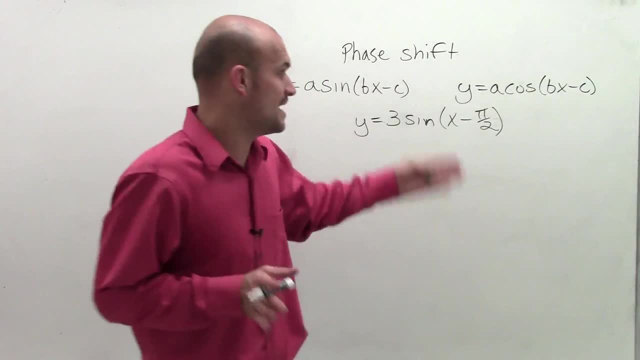 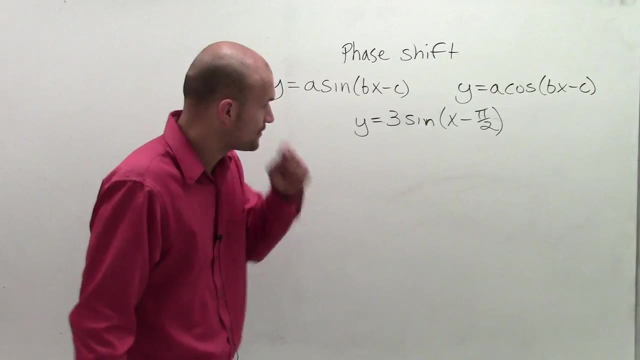 x minus pi over halves and, just like we've talked before, since that's negative, that's going to tell us to shift to the right. So we're going to take our whole sine function and shift it pi over 2 units. So what I want to do is I want to look at that. We know we can always do that when our 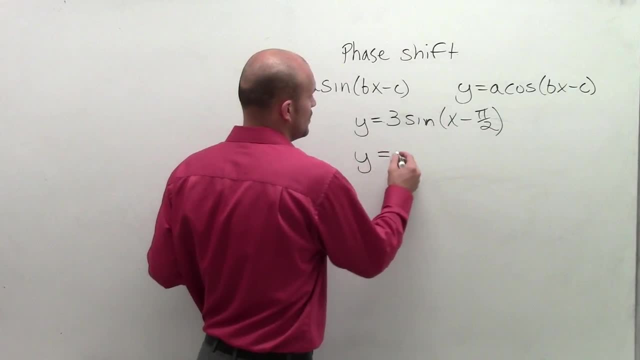 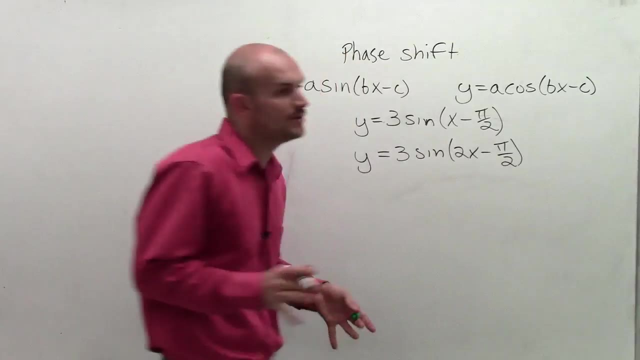 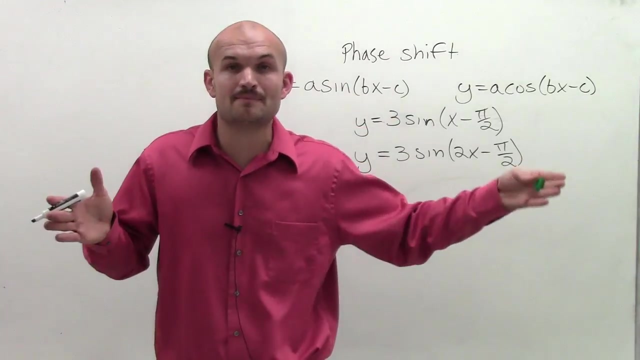 coefficient of x is 1.. So what happens when we don't have a coefficient of 1?? Well, that's actually going to affect our graph Because remember 2, that was your b right, And remember b affected our period And b was your period of how much you're going to compress or elongate. 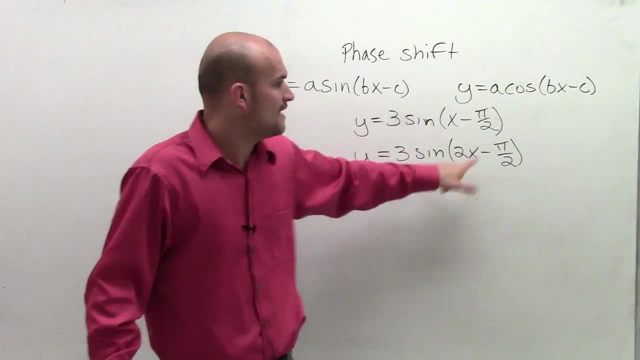 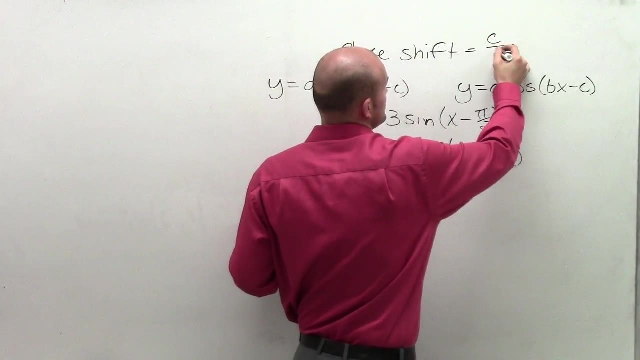 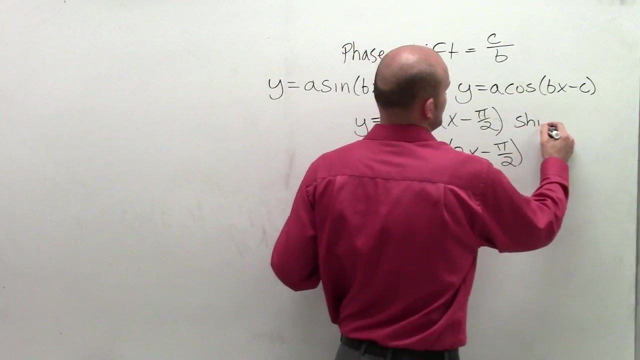 your function. So when we have a, b that's other than 1, that's going to affect our period. So our phase shift is actually equal to c divided by b. So let's take a look at actually our phase shift, Because in this example you could say you're going to shift pi over. 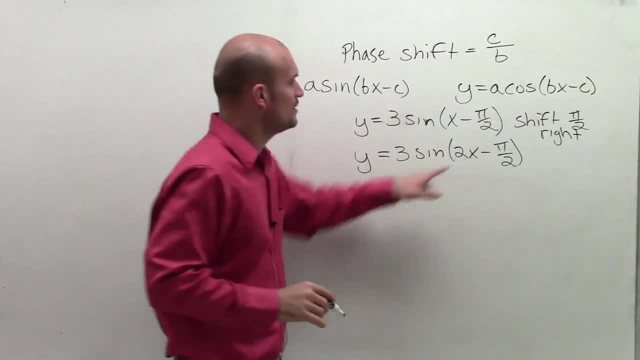 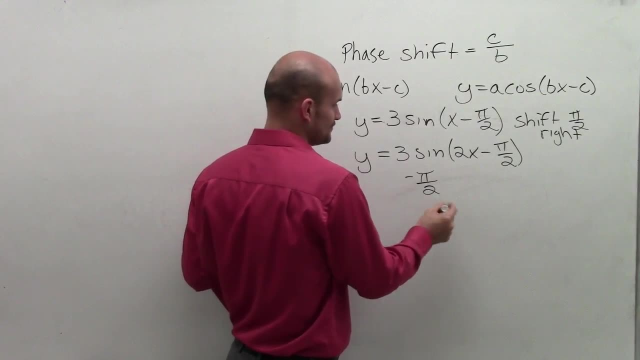 2 to the right. However, in this problem we need to make sure we take c and divide it by b. So I'm going to take pi- negative pi divided by 2, and divide it by 2.. And so I'm multiplying by the reciprocal. What I actually have is negative pi over 4.. So 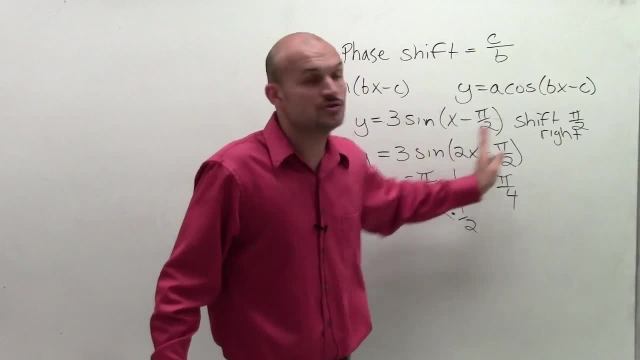 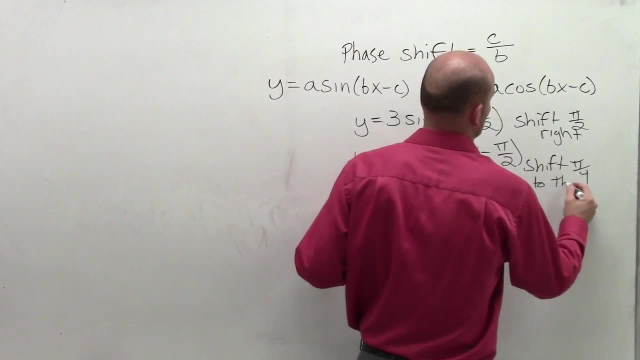 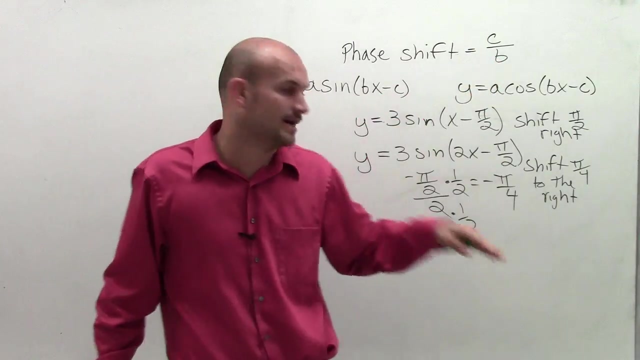 therefore, I'm actually, instead of shifting it pi over 2 to the right, I'm actually going to shift this graph pi over 4 to the right. So it's really important when you're dealing with phase shift that you understand. if there's a b other than 1, you have to make sure you 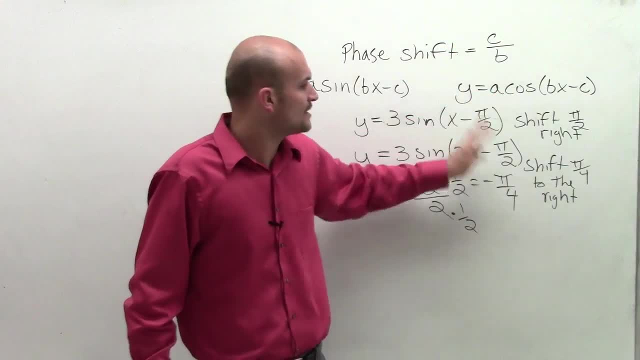 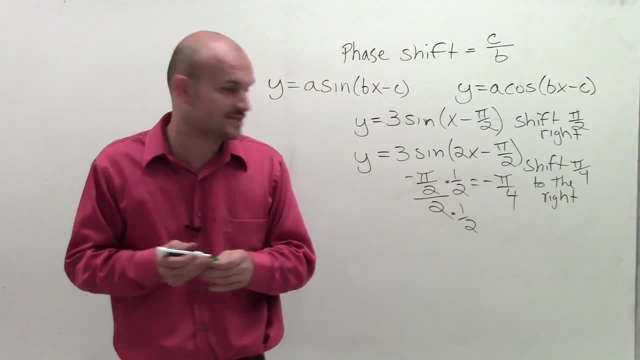 account for that phase shift By taking c divided by b. then what that value is going to tell you where to shift. it either left, if it's to positive, or right if it's going to be to the negative. So there you go, ladies and gentlemen. There's a quick little definition of your phase shift. Thanks,